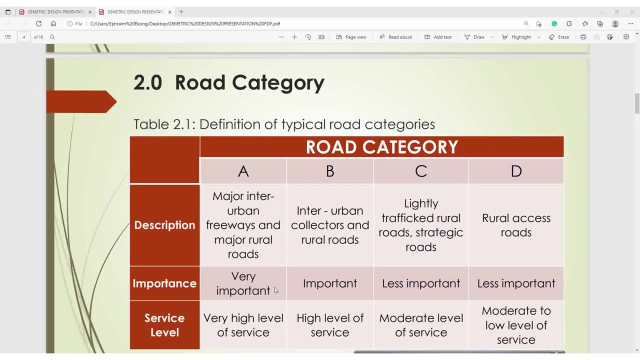 or category. As you can see, we have different road category цd. we have eight bay city on that category key. We have description Major into Urban Freeways and Major Rural Roads category cat Category in I. so we have description Major in inter urban free ways and major rural roads and major get切. 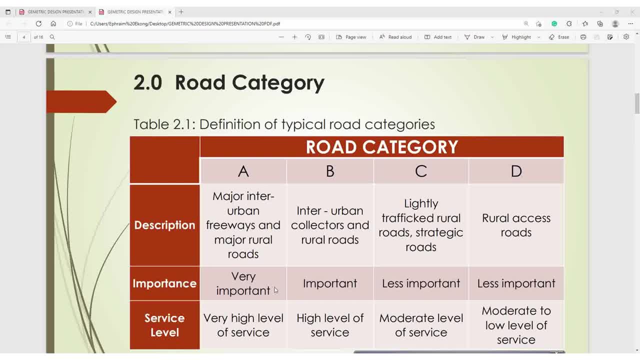 important Part물. Let's see different categories from your country. in here teams have autechımacy: Rural Roads. Category B- Interurban Collectors and Rural Road. Category C- Lightly Trafficked Rural Roads. Strategic Roads. Category D- Rural Access Road. Under importance of Category A. 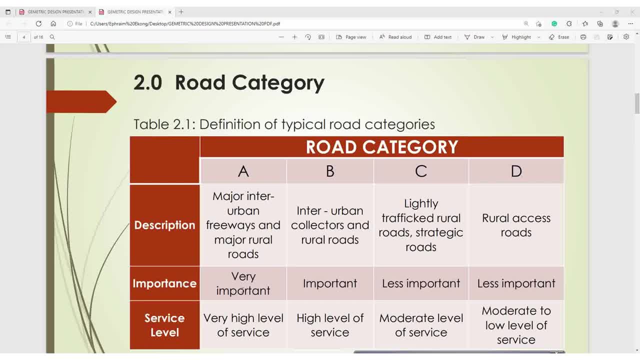 we have very important meaning. it's a very important highway. The traffic flow is high. Under B we have importance. It simply means the highway is of essence and it's important. We also have reasonable high traffic flow And under Category C we have less importance. 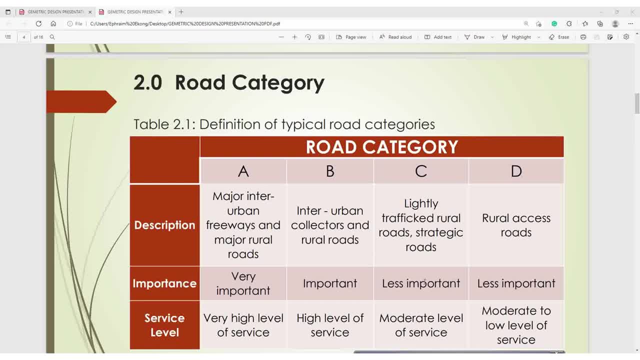 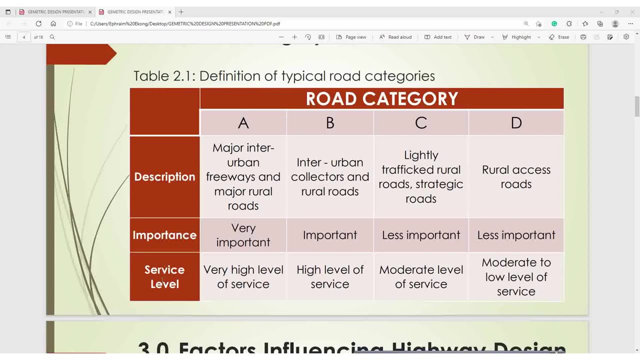 The highway or the road is important, but not as important as compared to Category A and B. Then Category D is also less important. So look at service level under Category A: very high level of service. Category B: high level of service as well. Category C: moderate level of service. Category D: 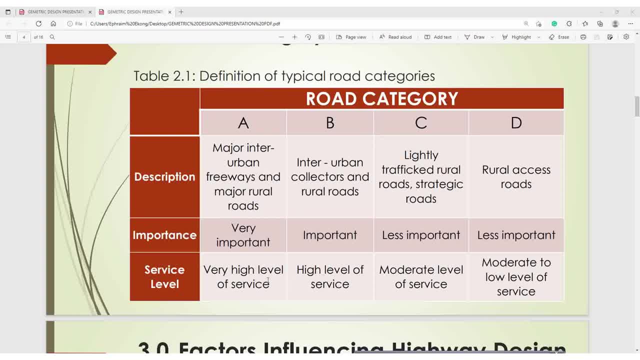 moderate to low level of service. So what this is trying to say is this road category: trying to say that Category A is a very, very important highway. The traffic is very, very high, Vehicle played, a road per second, per minute, per hour, every day, every day, every day. Category B also is an important 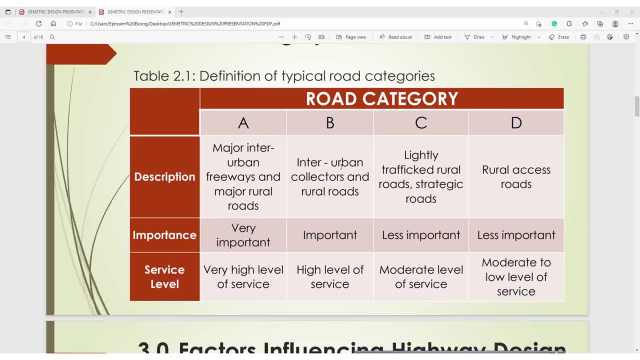 highway compared to C and D. So when designing your highway you have to know what type of road. Does it fall within Category C or Category B? Does it fall within Category E Or does it fall within the Appreciate Highway, modernityfectionc and just as a kind of excited troubled users? 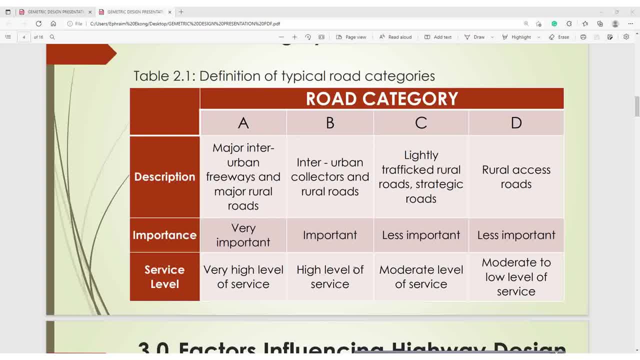 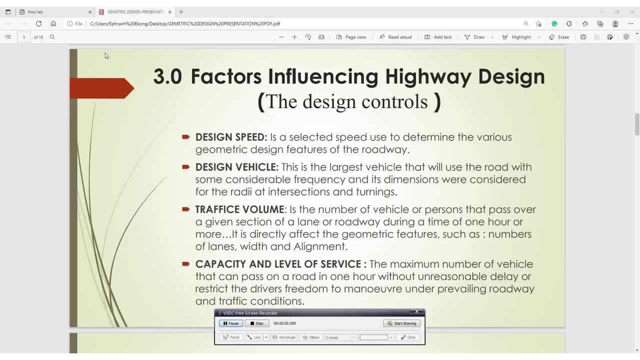 within category a, b, c and d. so you have to know all these before designing your highway. so we go to next one: 3.0. factors influencing iowa design. the factors influencing iowa design. they are also known as the design controls. what are these design controls? the design controls. 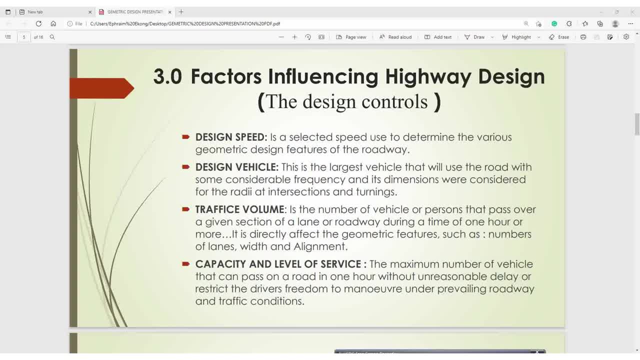 are the design speech, design vehicle, the traffic volume, capacity and level of service. the design speed is a selected speed used to determine the various- remember- design features of the roadway. so your design speed is important when carrying out your eu design. also, you could determine your design speed from root category, if it's category a. 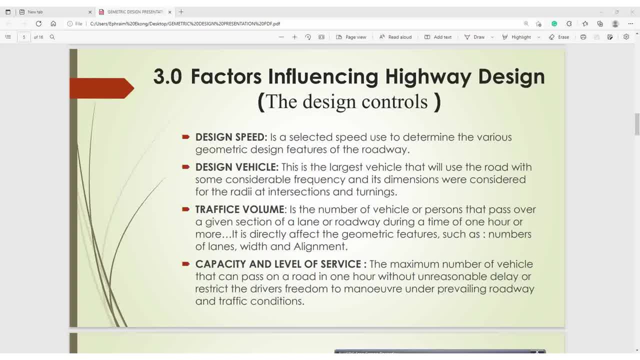 v, c and d of the design vehicle. this is the largest vehicle that will use the road with some considerable frequency and its dimensions were considered for the radar at intersections and turning so with your design vehicle, you will say, okay, fine, what is the design vehicle? is it a truck? is it a bus? 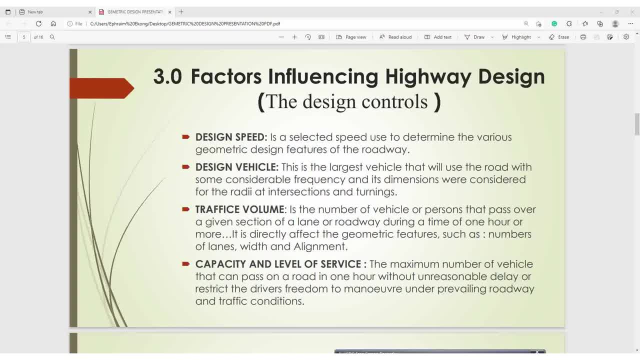 is it a passenger's car? so you, so you, should know what vehicle will use this road when wish you were designing what kind of vehicle from there, you could now carry out your design. traffic volume. traffic volume is the number of vehicle or price or person that pass over a given section of lane or roadway during a time of one hour or more. 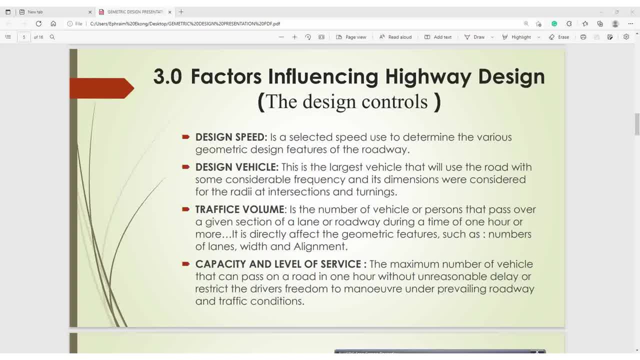 it is directly affects the geometric features such as number of lane, width and alignment. so your traffic volume directly affects the number of lane, the width and the alignment. so traffic volume is important in your design capacity and level of service. the maximum number of vehicles that can pass. 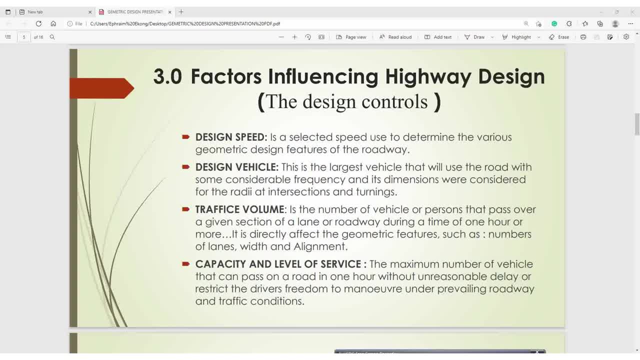 on a road in one hour without unreasonable delay or restrict the driver freedom to maneuver under prevailing roadway and traffic pollution. so this is your design controls. they are very, very important in your highway design, so you put them into consideration. we move to the next one. we also have factors replacing highway design. 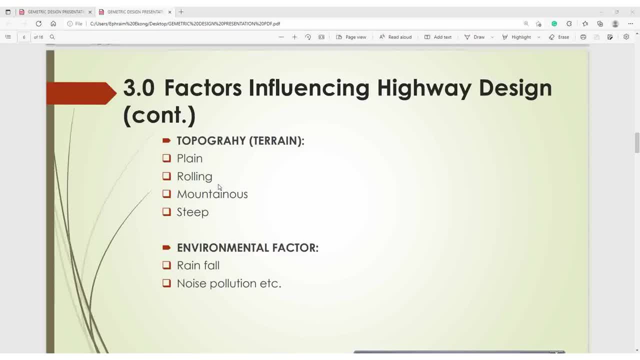 the topography and the environmental factors. under the topography we have the plane, the rolling, the mountainous and the steep. so if your topography is plain, rolling or mountainous, you have to put this into consideration because with this it could help you to emphasize your design speed and other. 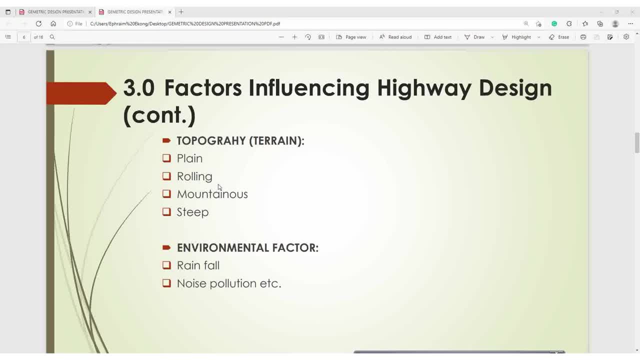 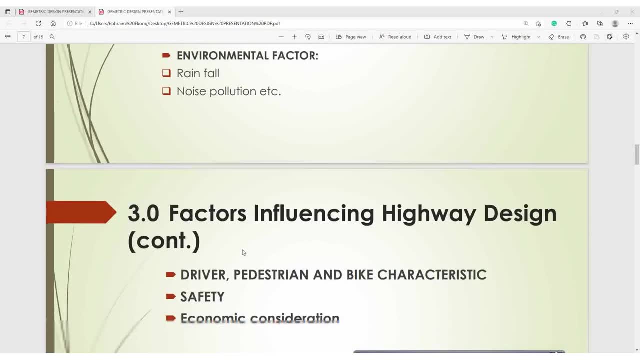 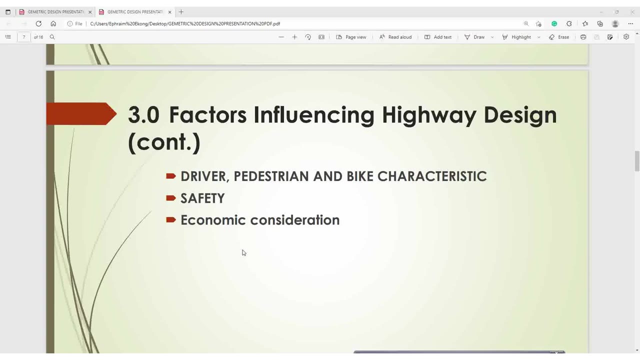 design controls needed in your design. we also have environmental factors, which are the rainfall, the noise, pollution, etc. on their factors influencing highway design. we have the driver, the district and the bike characteristics. we have the safety and economic concentration. so this is another key factors you should put into consideration. 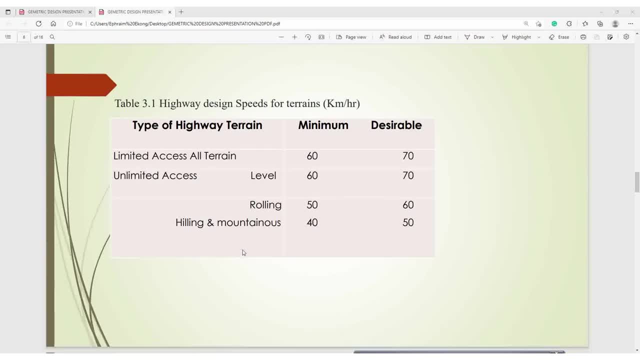 table 3.1: highway design. speed for terrain: kilometers per hour. so, as you can see your uh types of highway terrain, we have uh limited access, all terrain or limited access. we have level, rolling, healing and mountainous. so if your terrain is rolling, that is to say, 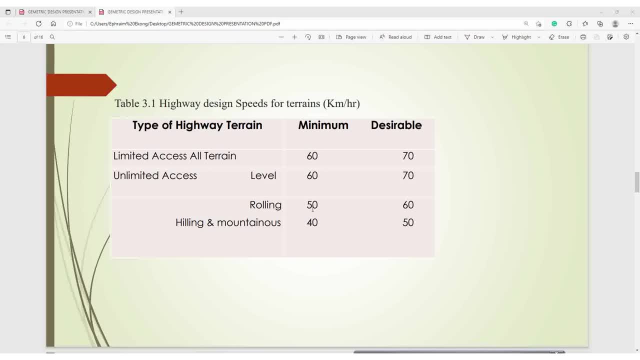 your design speed is it is either 50 or 60 kilometers per hour. so with this table you could emphasize: okay, my, my terrain is healing and mountainous so i could go for 50 or 40 kilometers per hour, as the case may be, as your design speed. so this table is gotten from federal ministry of works, iowa design manual. 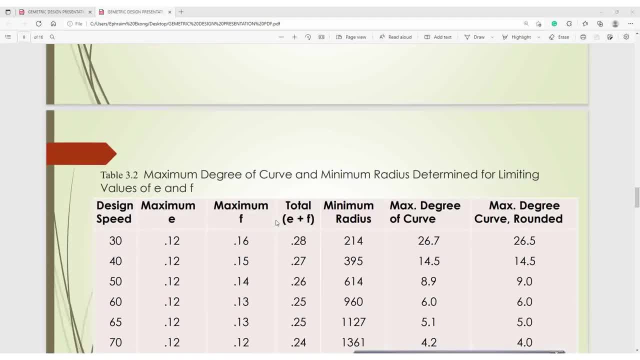 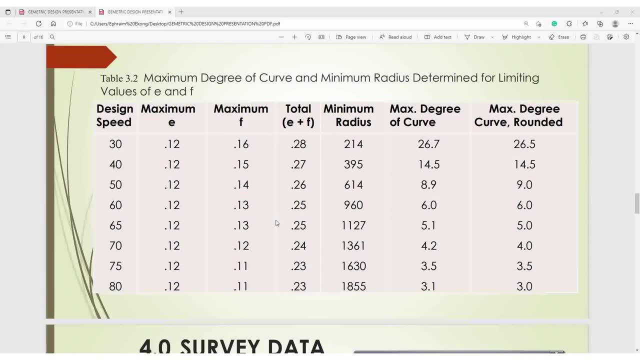 you can check it out. table 3.2: maximum degree of curve and minimum radius determined for limiting value of e and f. so our e here simply means super elevation, then f simply means our frictional force. so this is our design speed. we have 20, 40, 50, 60, so 65, 70, 75, 80, as the case may be. so if we have our 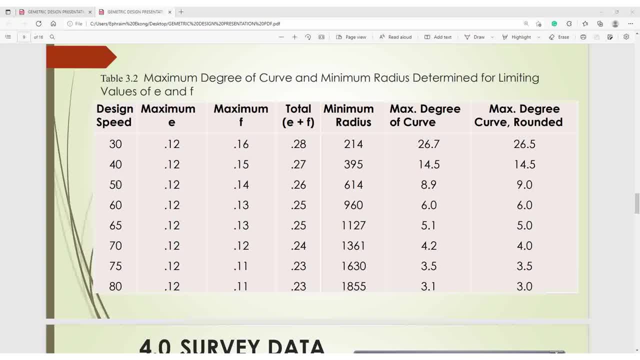 design speed to be 50. if we take it down, we have 614. so on that minimum radius, we have 614 meters. so if our design speed is 50 kilometers per hour, then our minimum radius should be 614. so that's how to get your design speed and your minimum radius. 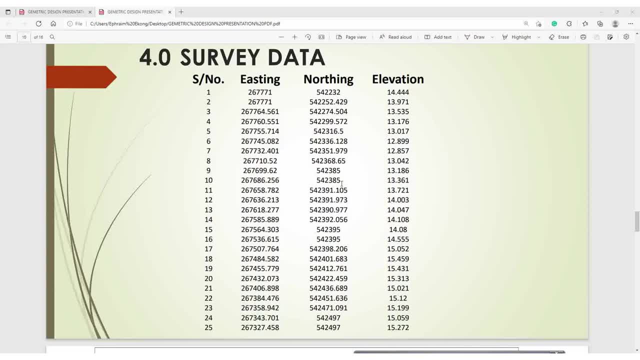 4.0 survey data. so this is a typical sample of our survey data gotten by the surveyor. so we have the easting and the nothing and elevation. when you impute this in excel and import it into civil trading software, it helps you to generate settings. 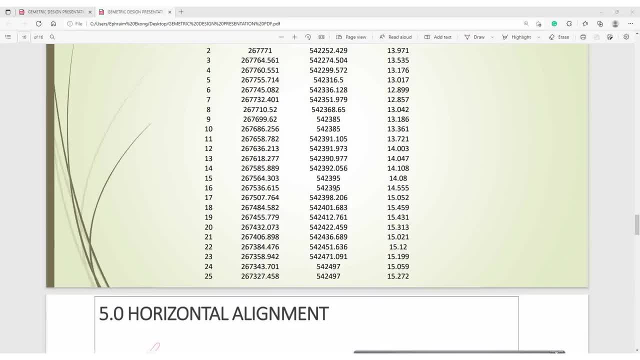 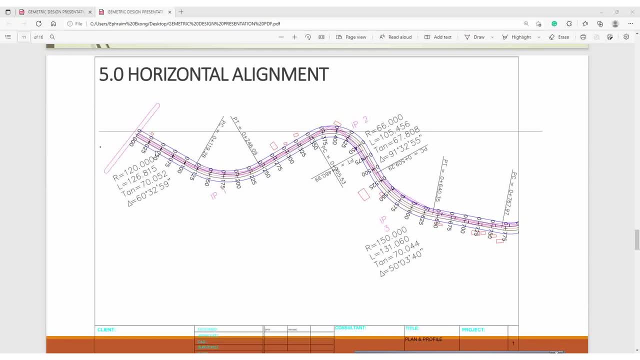 parameters such as your horizontal alignments. so this is your horizontal alignment. this is how it looks like it goes straight from chinese: zero, zero. it moves straight down. there's a curve here. now the essence of this curve, the major essence of this curve is is not um is to engage your driver. you don't make your driver get too comfortable. 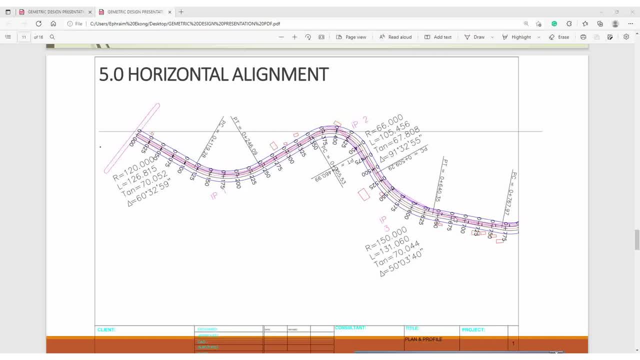 driving. so this is how the curve goes here. how simply means the radius, health, length of curve, our targets and our degree. the pc means points of curvature, the pt point of urgency. so this is a typical example of our horizontal alignment. the next is: so we have here our vertical. 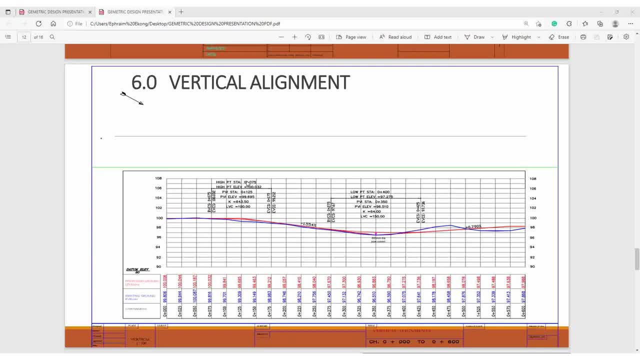 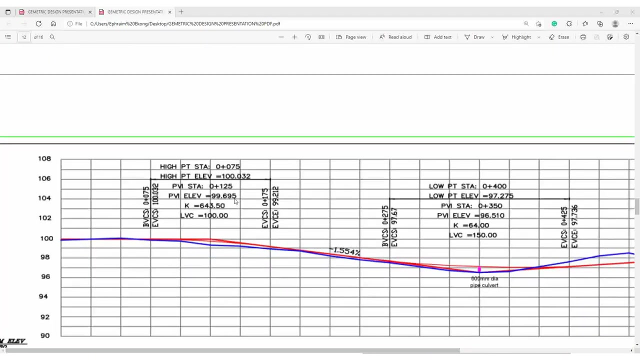 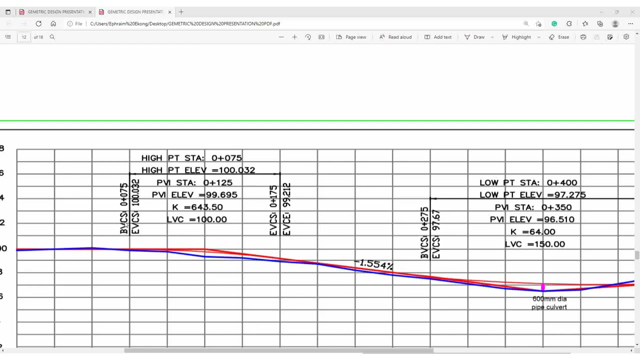 alignment, which is also known as our profile. so this red line is our existing ground on our profile. the blue line is our finished ground, our design level, finish round. that's upsetting key parameters here. this bvcs simply means beginning of vertical curve station, ending of vertical curve station. so this: 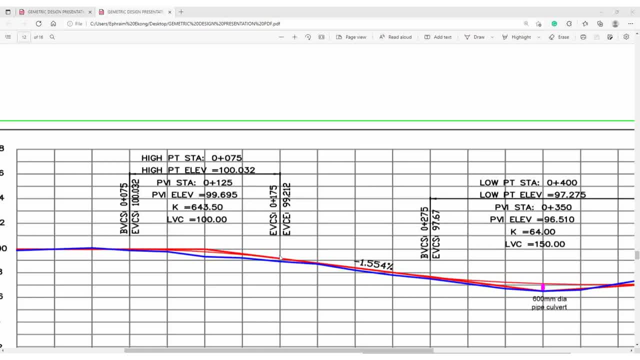 is where our vertical curve starts and this is where it ends. this is a criss curve. is a criss curve, is the criss curve here is ending of vertical curve station. ending of vertical curve. elevation point of ecstasy station, points of urgency elevation points of medical intersection point is this: 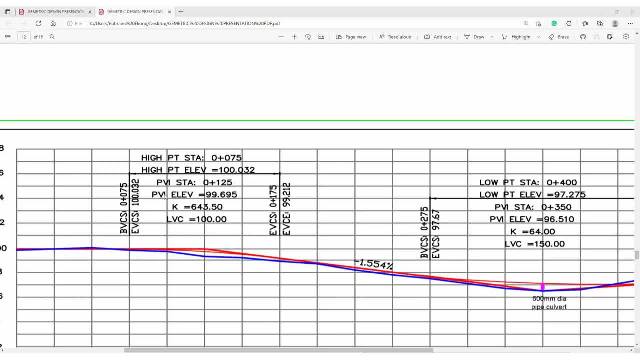 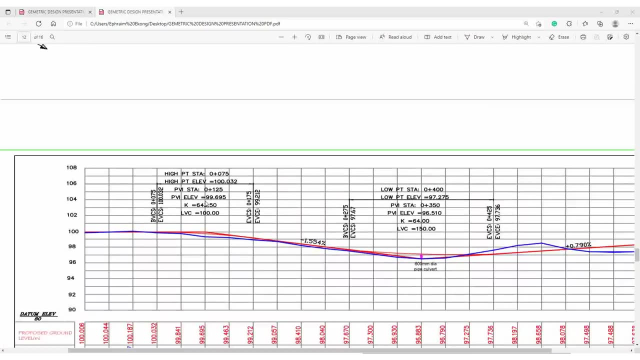 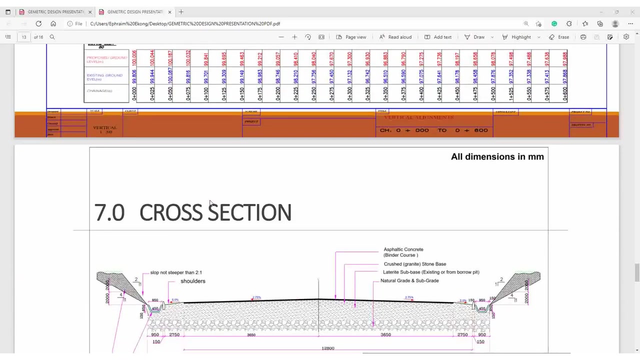 station points of a tiku isest intersection elevation. the K simply means vertical curve coefficients. LV- see- simply means length of rectangle length, length, length of vertical length, length of centrifugal length of vertical curve. so this is a typical example of our vertical alignment, also known as profile. the next is cross-section. the cross-section is a. 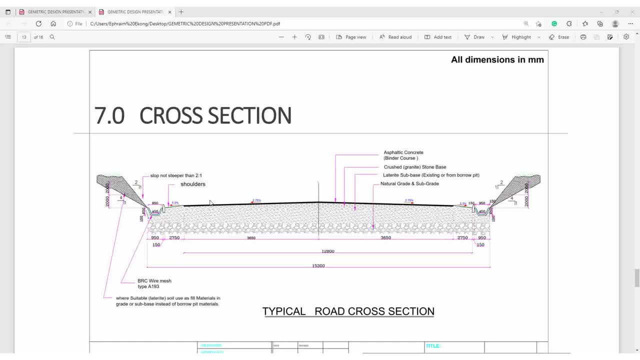 typical road section. this is how our typical road cross-section looks like. so two widths of the pavement is some point. three meters is three, six, three, six, five zero mm to left. three six five zero mm to the right. so this is our shoulder, this is our drainage. Travis water drainage: here is our natural. 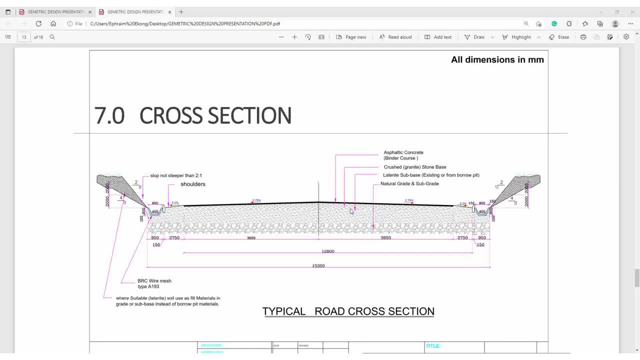 ground level. then here is a large rights of base existing or from Bo Peet's. next is crushed granite stone base and lastly is our- this one is as frantic concrete- the binder course. so this is a typical example of cross-section of our highway. so this is how it looks like. 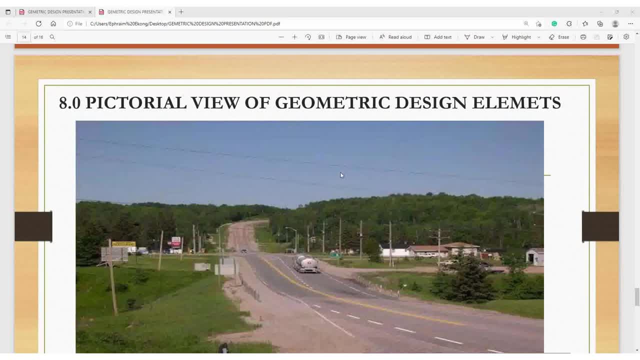 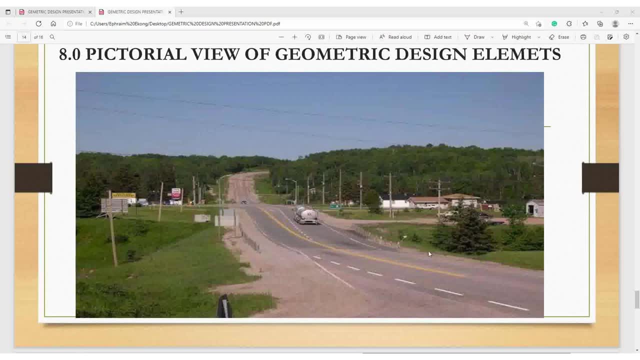 the next is pictorial view of commercial design elements. so this is our highway, this is the with in the beach, possibly maybe some point three meters wide and this is the curve. so you ensure you introduce the curve at some point they make. your essence of this curve is not to make your driver so